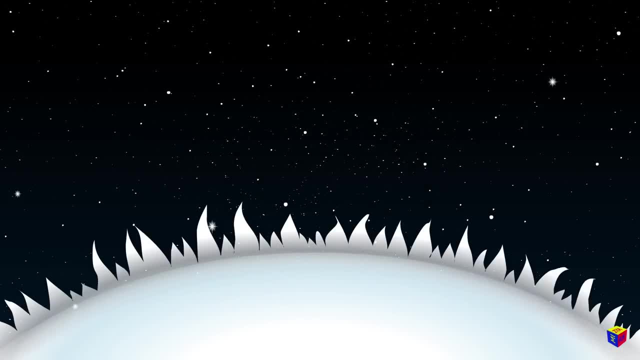 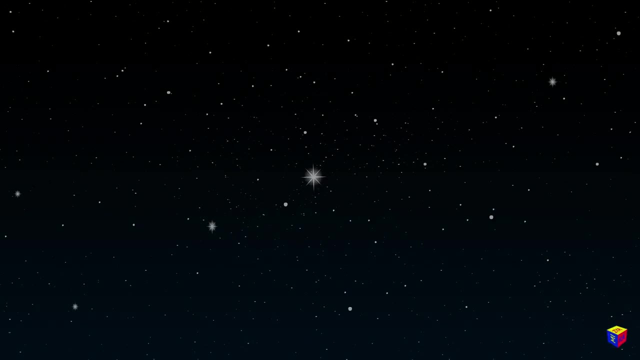 As a result of this burning, an enormous amount of light and heat is thrown into space. We see stars as tiny dots only because they are so far away from us. In order to get to even the closest star, not counting the Sun, we would have to fly. 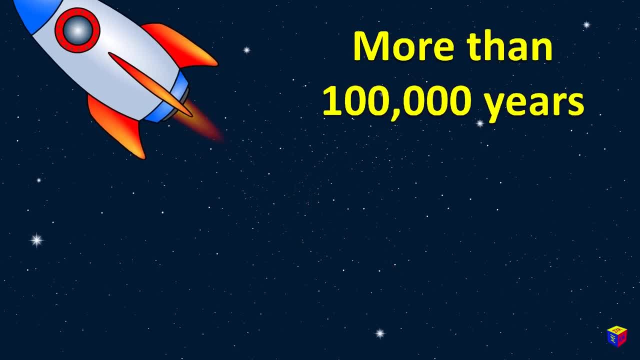 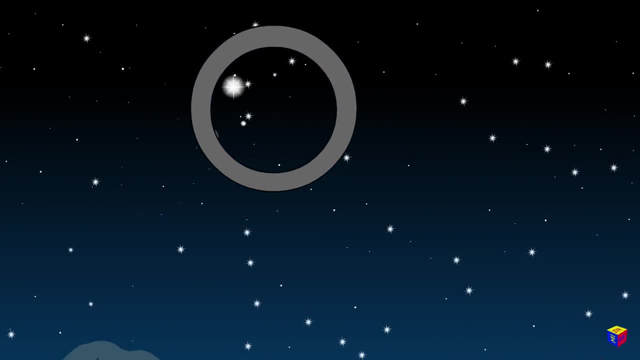 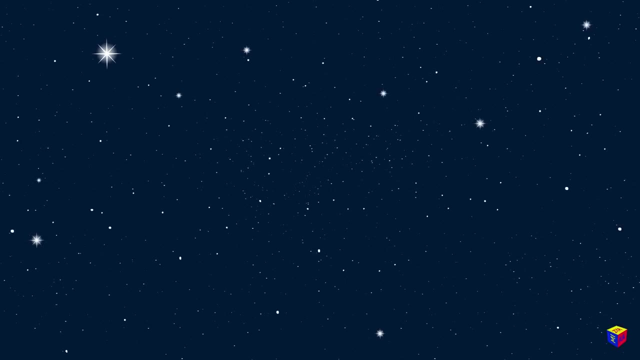 for more than 100,000 kilometers, That's more than 4,000 years. Stars differ in size, brightness and color. Also, the stars can vary in temperature. Blue stars seem to be cold, but in fact they're the hottest ones, with a temperature of more. 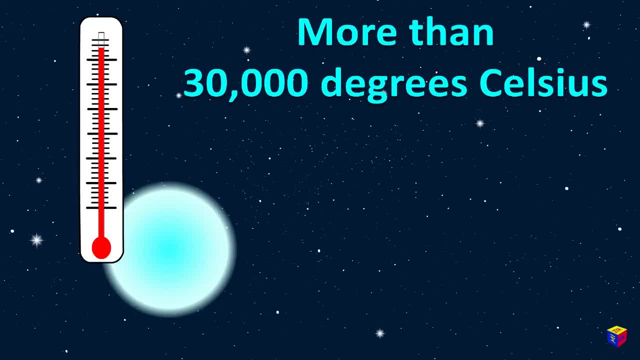 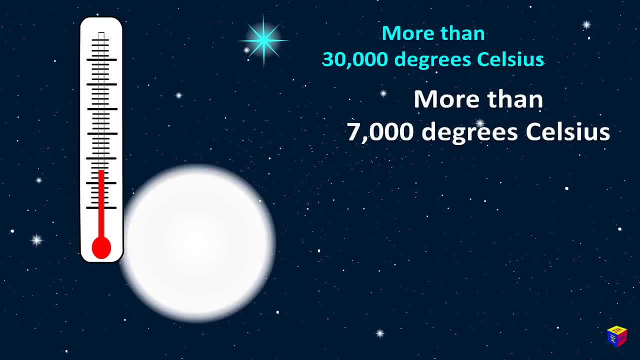 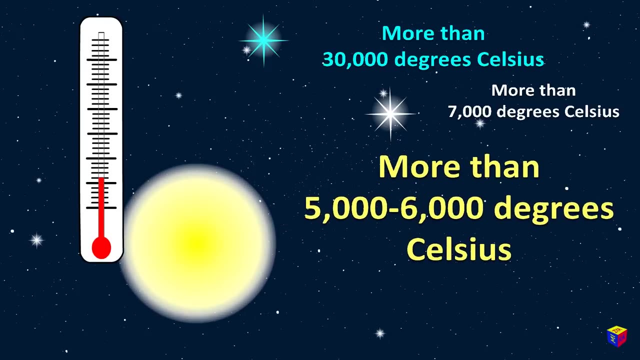 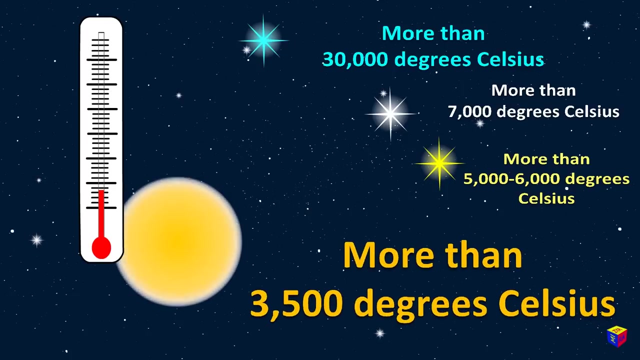 than 30,000 degrees Celsius. White stars are a little cooler. Their temperature is more than 7,000 degrees. Yellow stars have a temperature of 5 to 6,000 degrees, Orange stars more than 3,500 degrees. 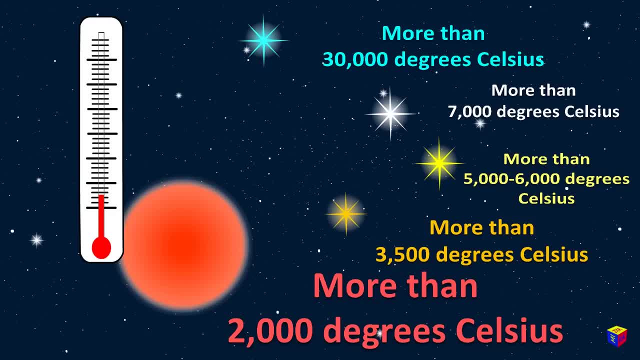 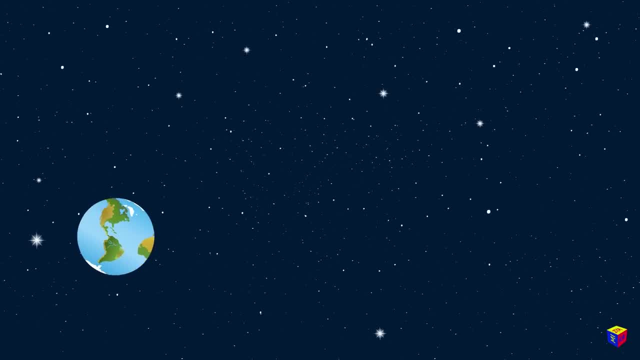 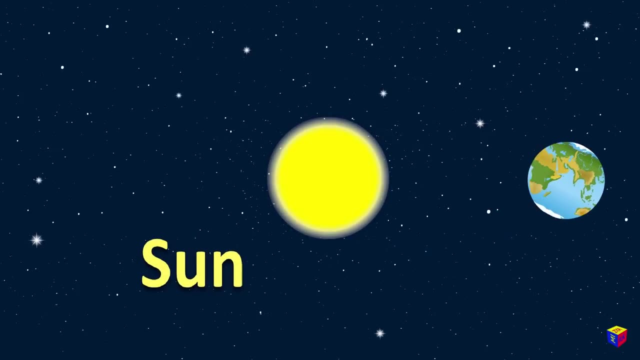 Finally, the coldest stars are the red ones. Their temperature is more than 2,000 degrees. Do you know which star is closest to Earth? Of course, this is our Sun. The Sun is a yellow star and its temperature is about 6,000 degrees. 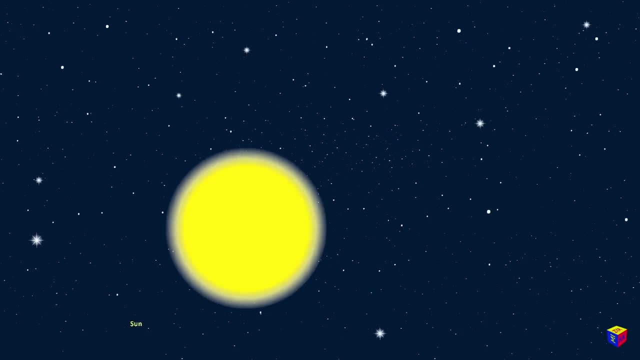 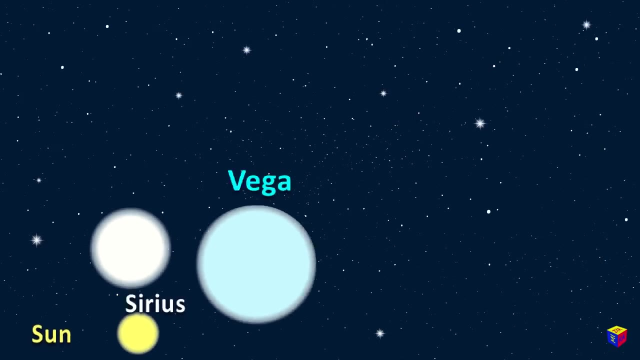 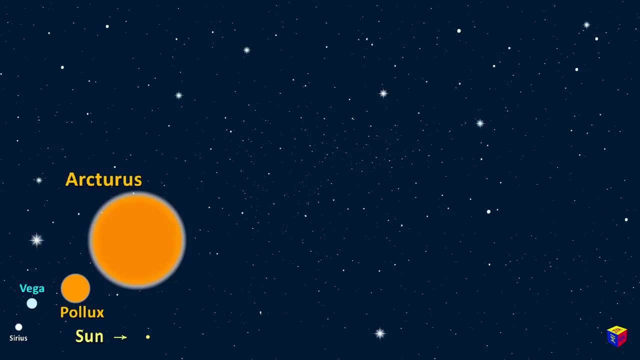 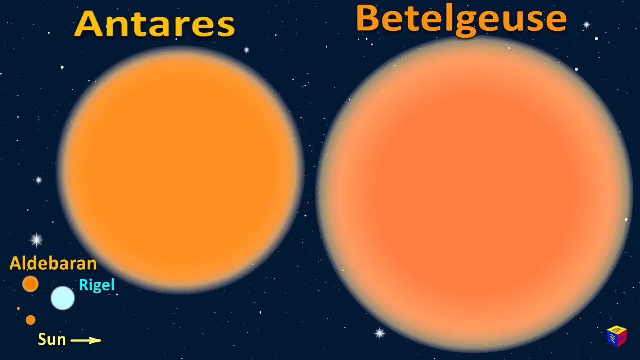 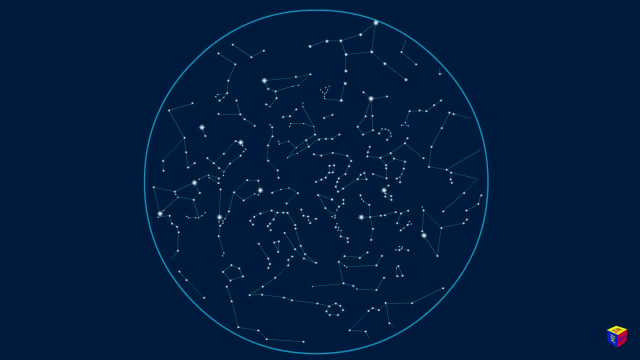 And this is how the Sun looks in comparison to some other larger stars: Sirius, Vega, Pollux, Arcturus, Aldebaran, Rigel, Antares, Betelgeuse. In ancient times, while observing stars, people grouped them into patterns called constellations. 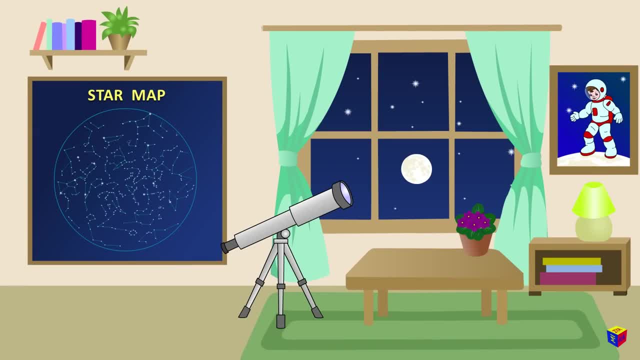 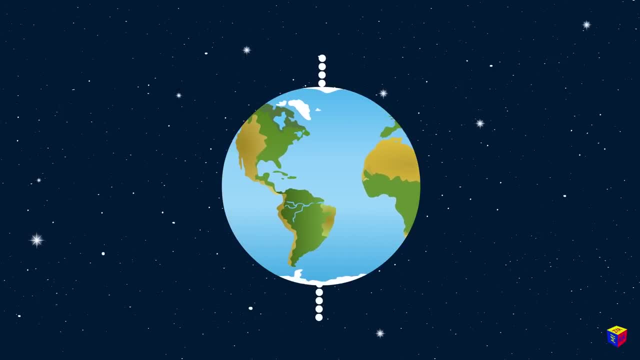 These constellations form a star map. Since the Earth is a star map, the stars are called constellations. Since the Earth is a star map, the stars are called constellations. The Earth rotates around its axis. The stars seem to move across the sky.